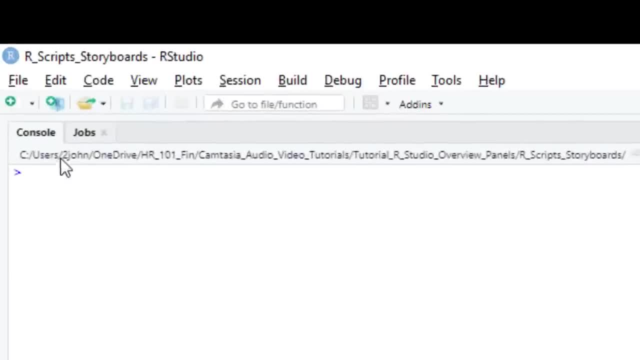 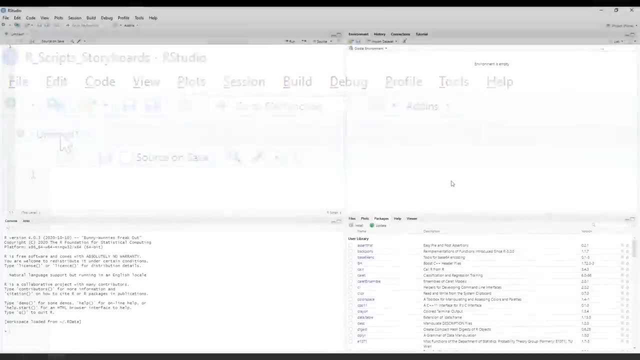 open. You can create a new script by going to File, selecting New File and then Our Script, And that will give you a new script in your source panel. Together, you'll probably spend around 99% of your time in the source. 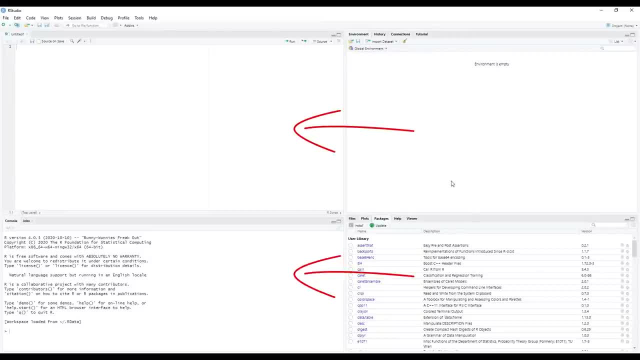 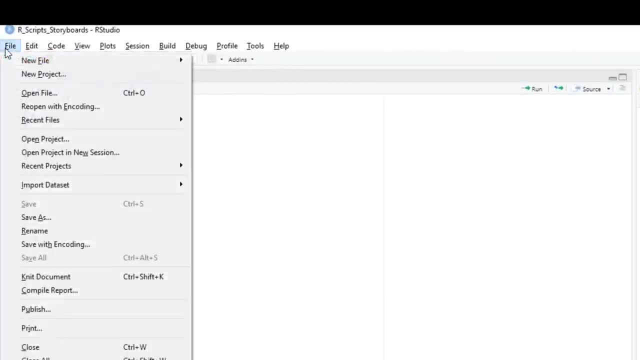 and console panels. so let's step through a simple example to show you how to work on those panels together. First we need to create a new script file. so we go up to our File menu, go to the first option which says New File, then select Our Script, just as we did before. 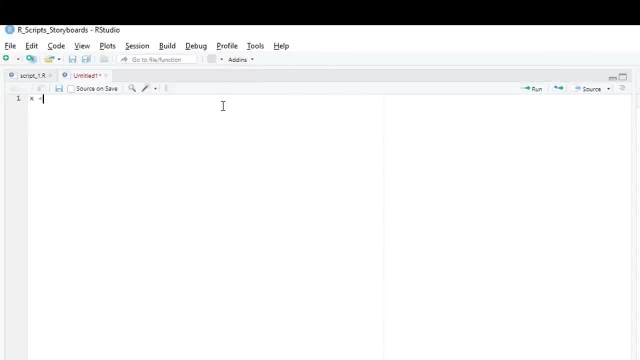 Now I'm going to just create a simple variable, which I'll call x, and assign it the values of 1 through 100.. I'll also create a second variable, y, which will be the cumulative sum of each item. I'll also create an element of x using the cumulative sum function. 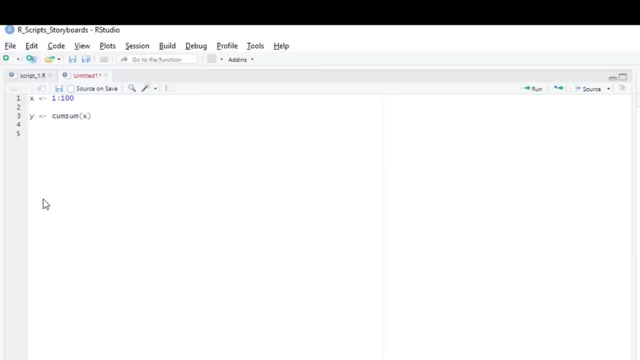 Now that I've written something, I want to save it. We can go up to the File menu and select Save, or we can just do a little Ctrl-S like we would with any other standard program. Okay, so now we have something written and we've saved it. 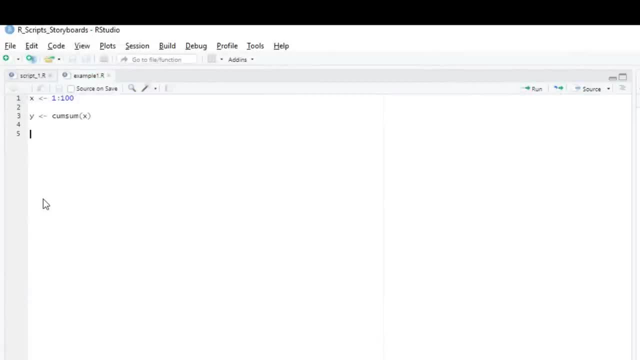 but R still hasn't run anything yet. We have to tell RStudio to run the code before it will do anything with it. To run our script, we just highlight the lines we want to run, go up to the Code menu and select Run Selected Lines. 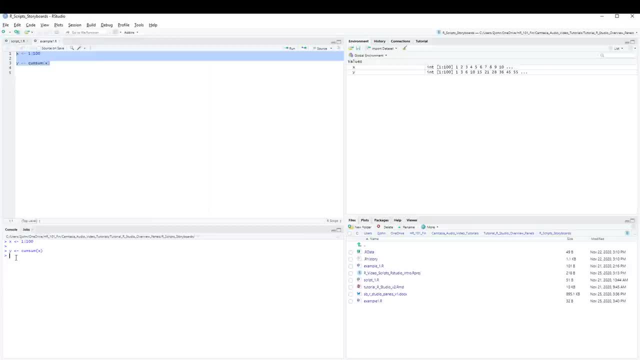 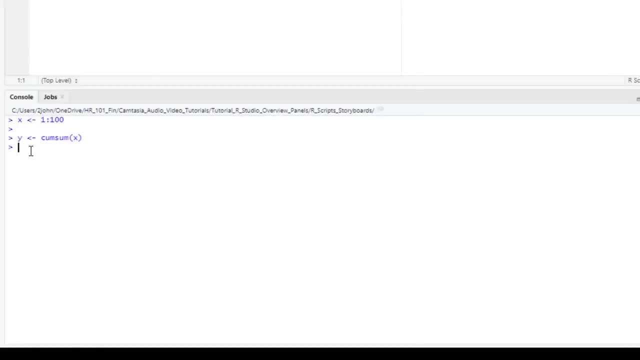 When we do that, voila, our code is run. I want you to first notice that we see our executed code down here in the console panel. In fact, I can now go directly into that console window and work interactively with those variables. For example, I can get the first six elements of our y. 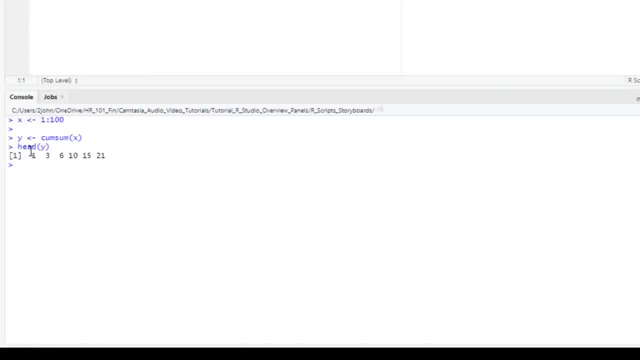 variable. with the head function I can also create new variables in the console. I will create a new variable, z, and assign the value of the median of y. When I type z in the console, I get my result. So big picture summary here. Use the source panel for scripting when you want to save your R code. 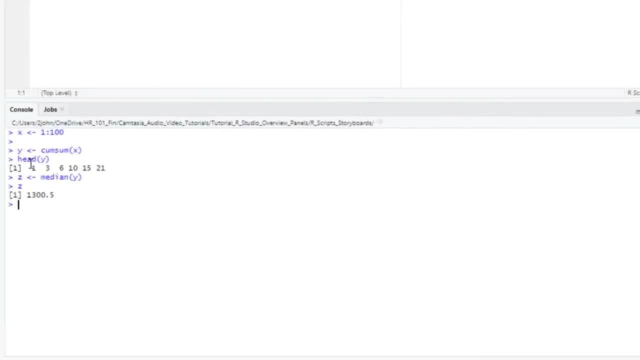 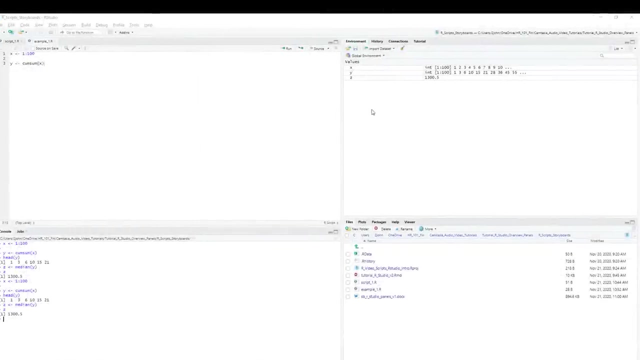 and run the commands again later. Use the console panel when you want to work with your data interactively. Now that you have a feel for the source and console panels, let's go to the environment panel on the upper right. You'll notice that this panel is showing the variables we just created. 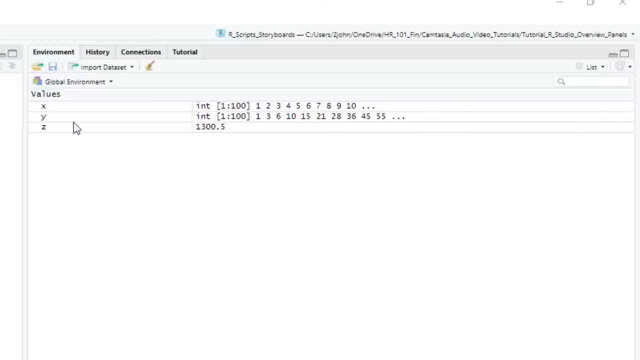 including that z variable that we created in the console. This shows us the name of the variable as well as some information about the object, like it's an integer vector of length 100.. If we want to start off with a clean environment, we can just click. 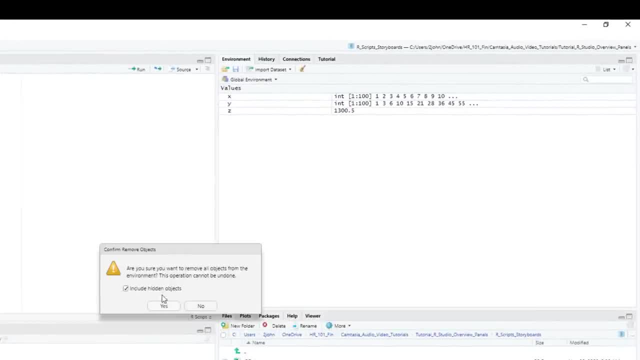 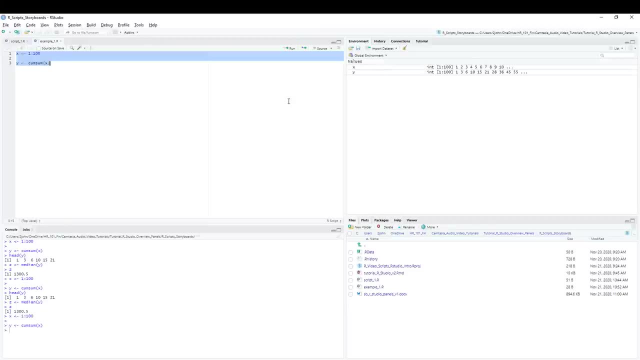 the little broom here say yes, that we're sure we want to get rid of everything and then we'll have a clean environment. If we want to get those variables back, I just go back into my script highlight and run those lines. this time I'm using the control enter. 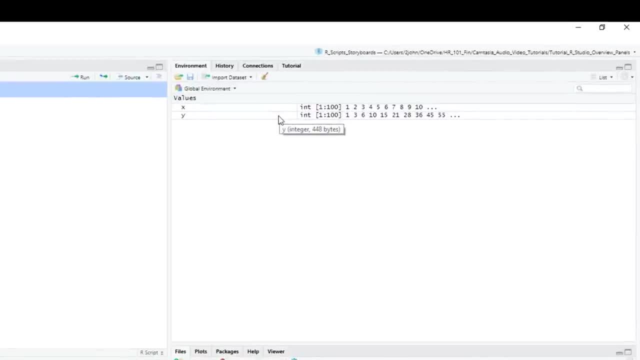 shortcut and see that we have those values back in our environment, Although notice that that z variable won't be there because, remember, we created it interactively rather than as part of our script. There are some other tabs here too, including the one for importing data, which I would encourage you to explore on your own. but the environment. 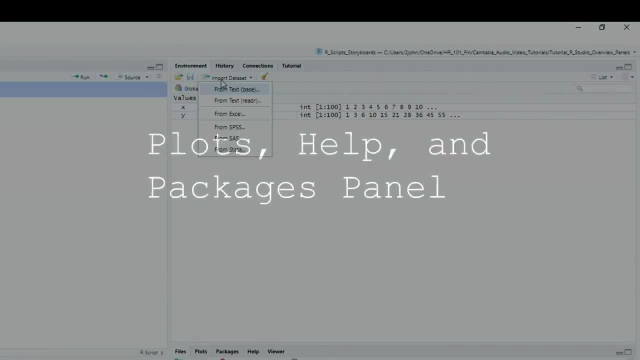 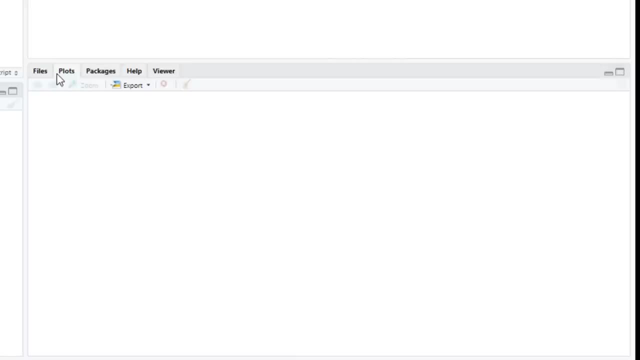 tab is really the only one that I use regularly. Now let's move to this panel on the lower right, which has several different tabs. We'll start with the plots tab, which shows us the results of any plot we make in the source panel or in the console, For example. I'm going to 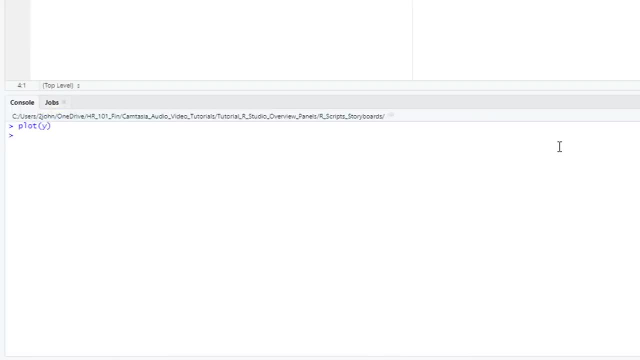 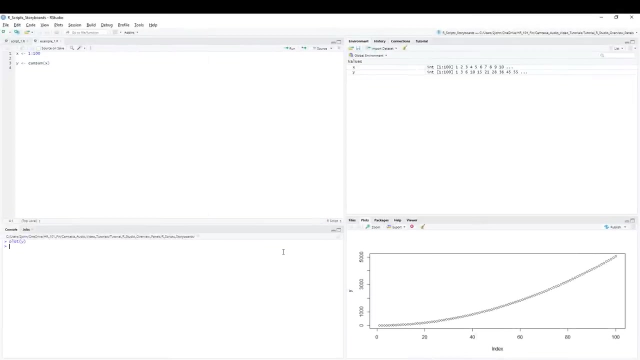 go to the console and plot my y variable, which was the cumulative sum of the x values. When I do that, I see the results in the plots tab. If I make a new plot, say plot x, you'll see the new plot there too. 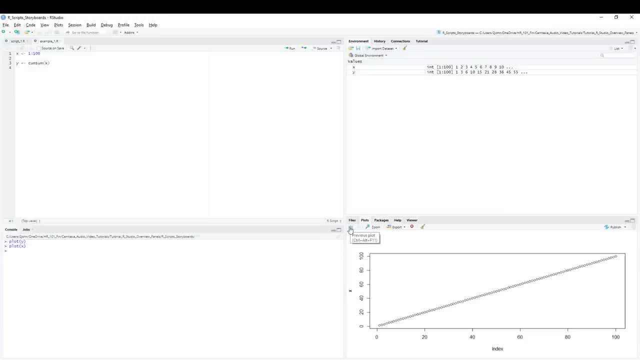 If we want to go back and look at the previous plot, we can just click on the little arrow. You can clear these plots just by clicking on the little broom. If these are plots that you want to run again later, you can put these commands in the script and then run them from there instead, And again you'll see. 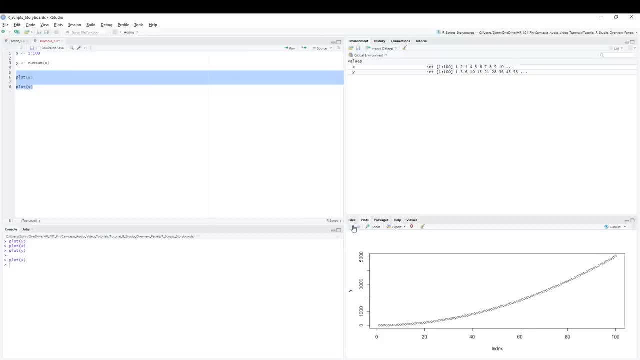 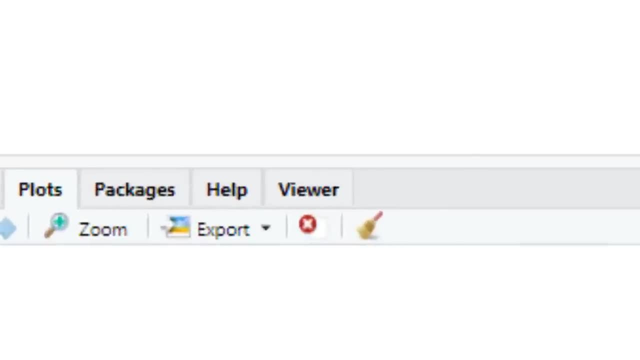 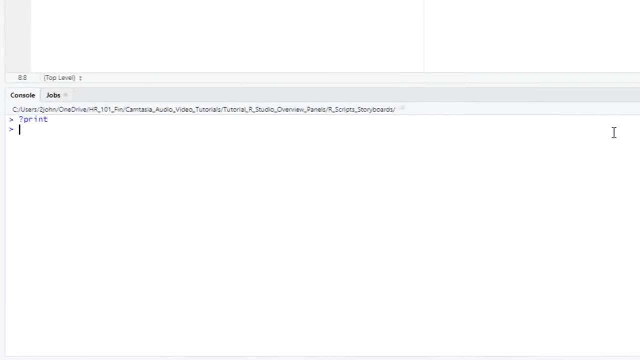 them pop up in the window. We also have a help tab which shows us the results of our help queries, which we can get just by putting a little question mark on the top right corner. For example, if I go down to the console panel and I type print to get help on the print function. 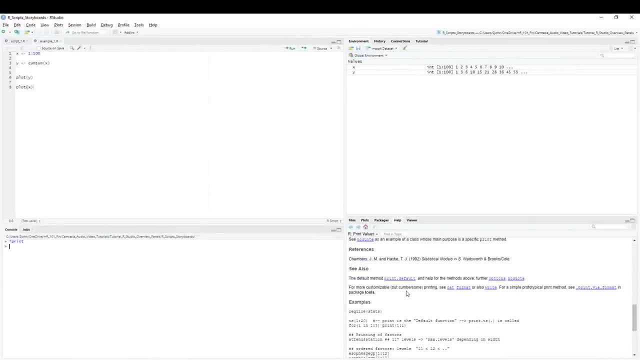 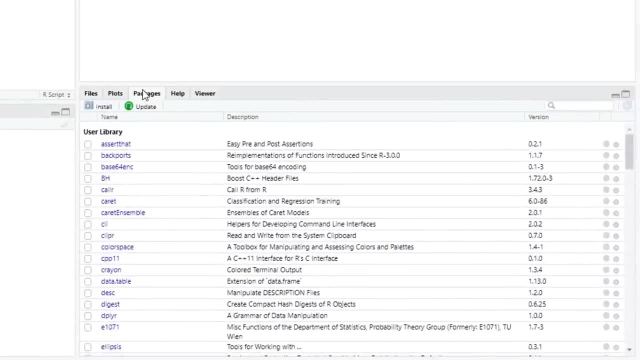 my tab switches over to help and shows me all kinds of information about the print function. Finally, we'll take a look at the packages tab. As a reminder. the real power of R is a large set of libraries- over 10,000 at this point- each containing specialized functions to help you.